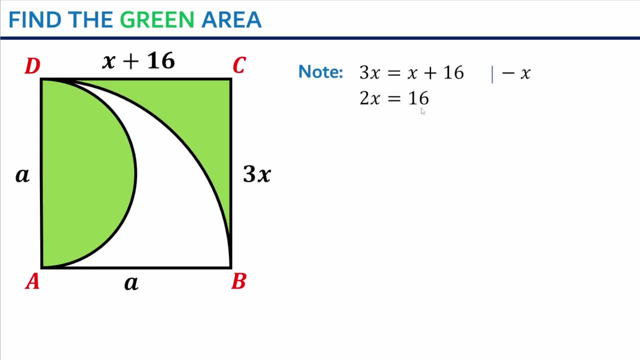 x is equal to 16.. And if we divide both sides of this equation by 2, we get the equation x is equal to 8.. So x is equal to 8 and we know that the square has a side length of 3 times x is equal to. 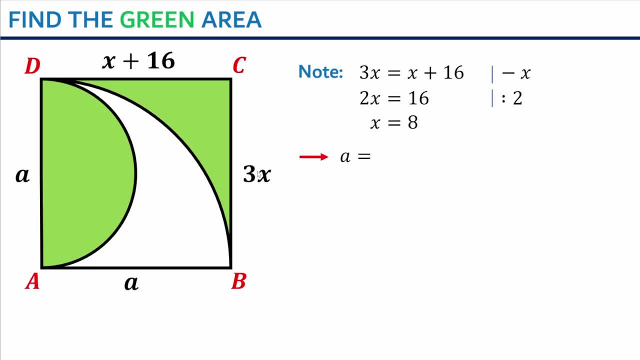 the side length of 3 times x. This means that the side length of the square is equal to 3 times 8, and 3 times 8 is 24.. So our square a, b, c, d, has a side length of 24.. 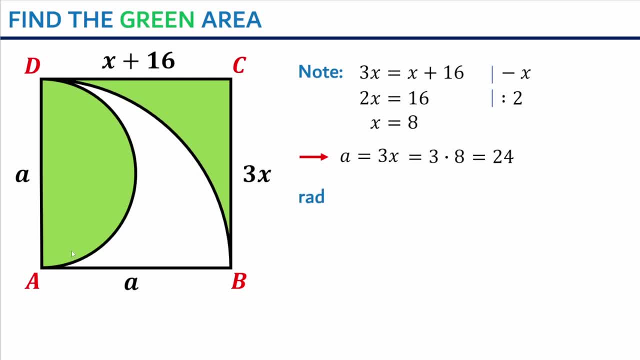 Now let's have a look on the semicircle. We know that the diameter of the semicircle is equal to the side length of the square. So the semicircle has a diameter of 24 and the radius is 1 half times the diameter. 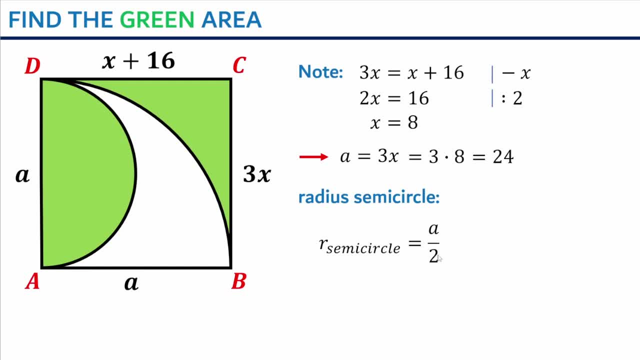 So the radius is equal to 24 divided by 2, and this is equal to 12.. So our semicircle has a radius of 12.. The radius of the quarter circle is equal to the side length of the square, So our quarter circle has a side length of a. 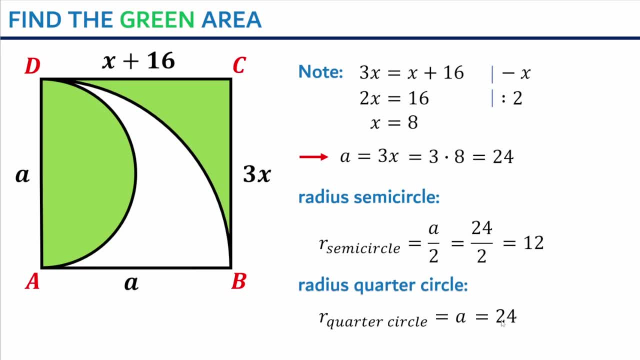 And a is equal to 12.. So our square a, b, c, d has a side length of 24 and the radius of the semicircle is equal to 24.. Okay, now we can easily calculate the green shaded area. as we already mentioned the 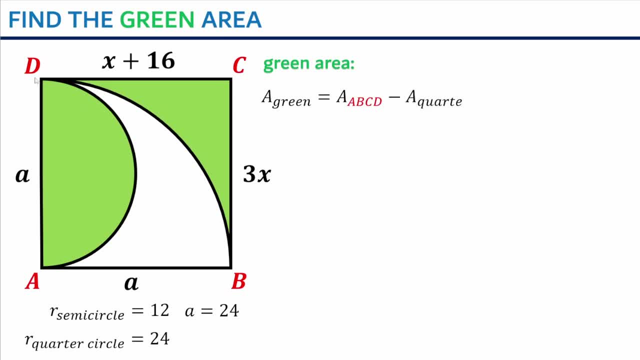 green shaded area is given by the area of square a, b, c, d, minus the area of the quarter circle, plus the area of the semicircle, The area of square a, b, c, d is equal to the square of the side length. 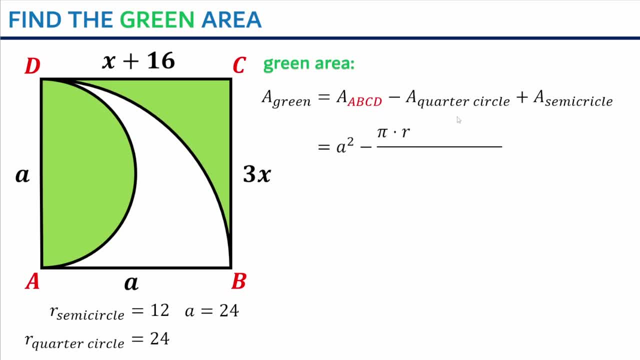 The radius of the quarter circle is equal to the side length of the square divided by 4.. The area of the semicircle is equal to the side length of the square divided by 2.. We know that a is equal to 24..